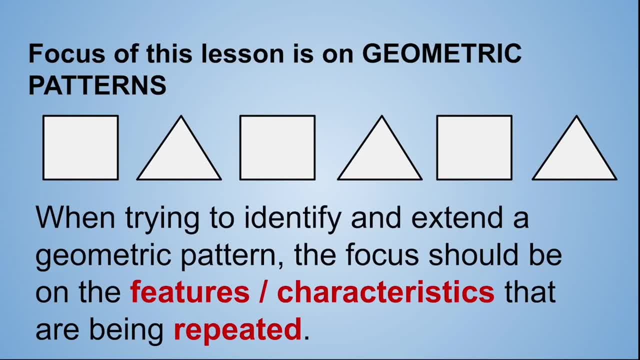 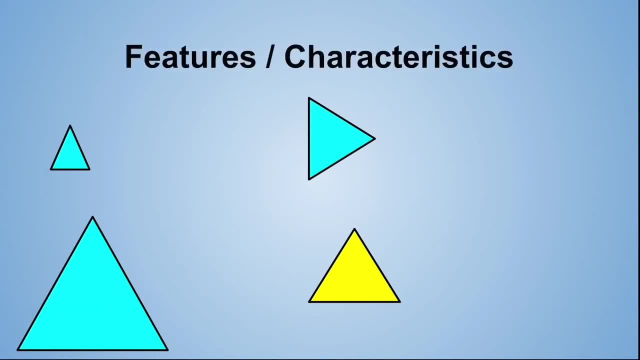 that are being repeated. Let's talk about the different features or characteristics that help us to identify and extend a geometric pattern. Our first characteristic is shape, and we have an example of a triangle. Our next characteristic is size, and we have a large triangle as an example. Then we have direction, an example of a. 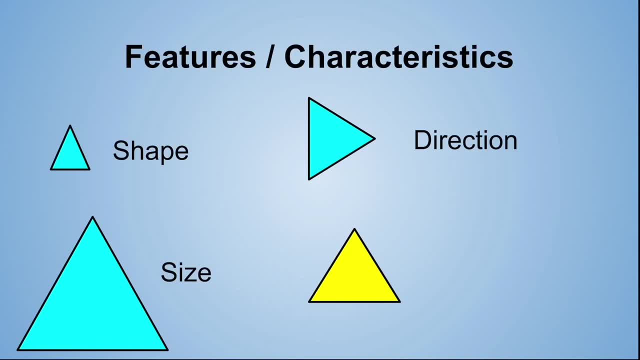 triangle that is pointing towards the right-hand side. Our last characteristic is color, And here we have an example of a triangle that is yellow in color. So Go3s always remember the characteristics or features that help us to identify and extend a geometric pattern, And these characteristics are shape, size, direction and color. 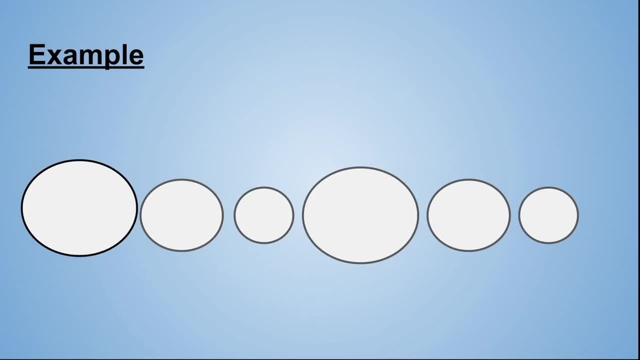 Let's have a look at this example of a geometric pattern. In this geometric pattern, only one characteristic is changing. Can you tell me what characteristic this is? The characteristic that is changing is size. First we have a large circle, then a medium. 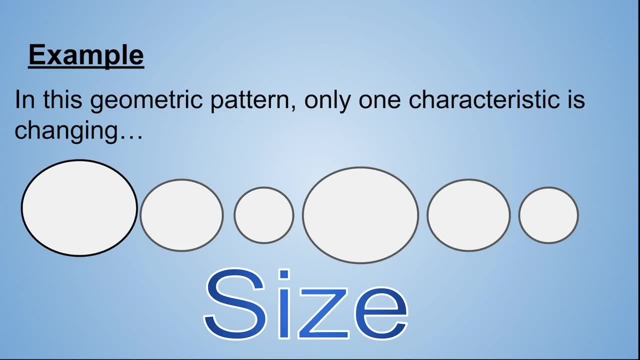 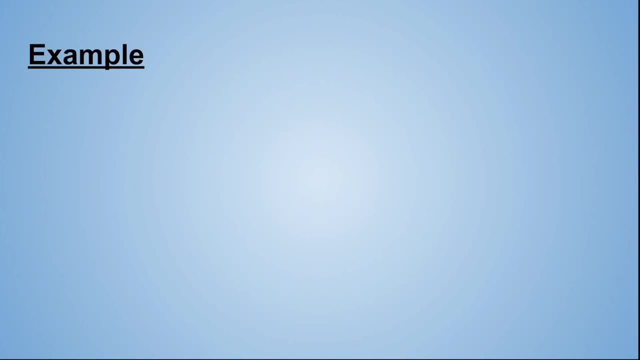 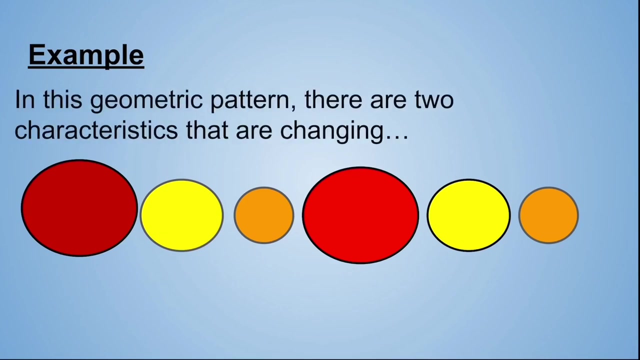 circle, then a small circle, then again a large circle, a medium circle, then a small circle. Let's have a look at our next example of a geometric pattern. Let's have a look at our next example of a geometric pattern. In this geometric pattern, there are two characteristics that are changing. Can you tell me what these? 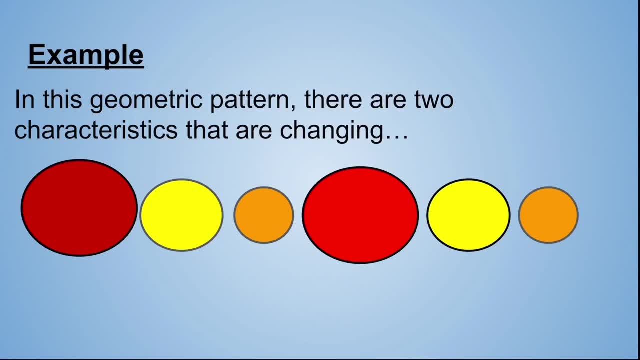 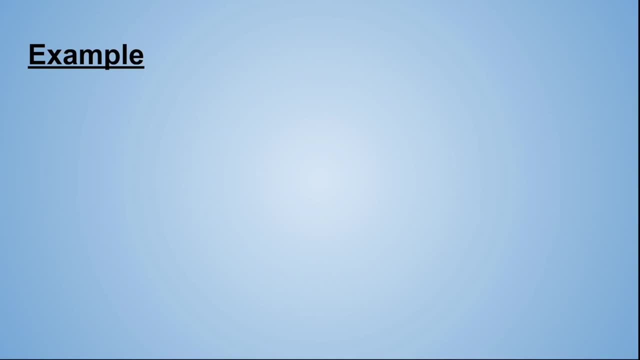 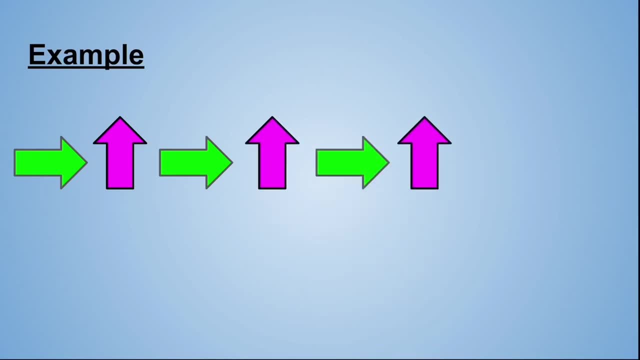 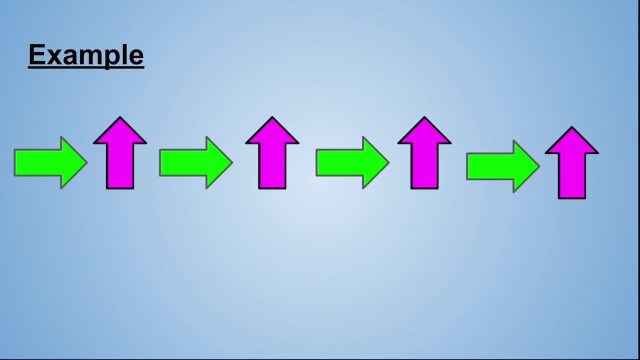 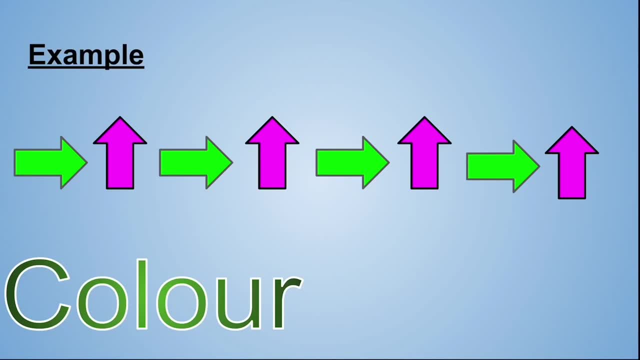 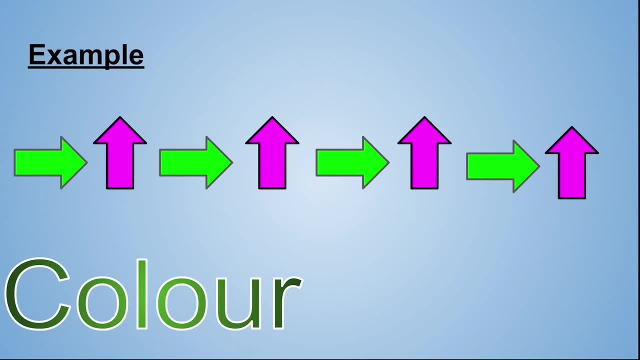 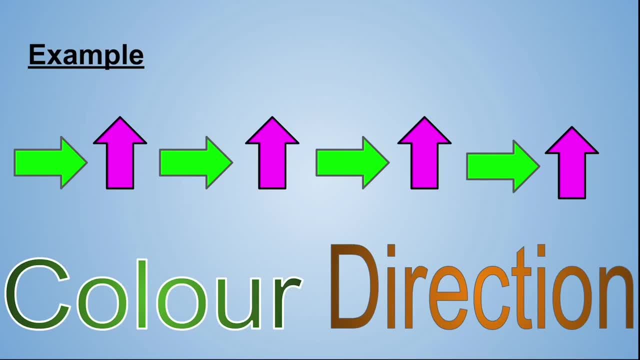 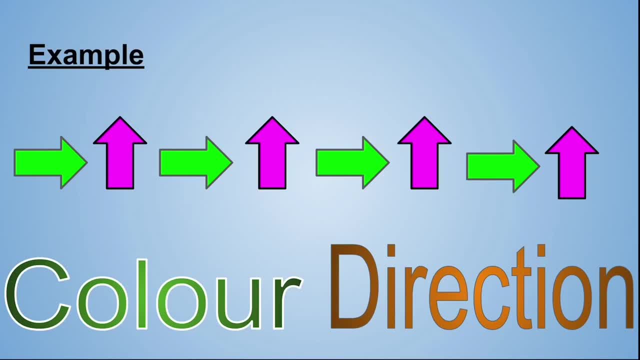 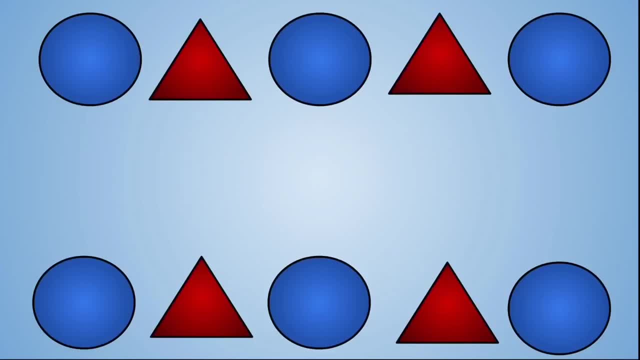 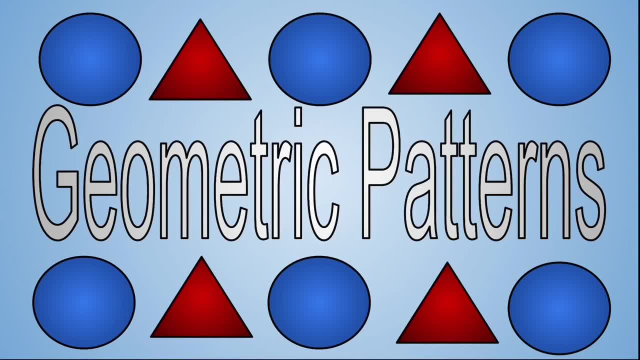 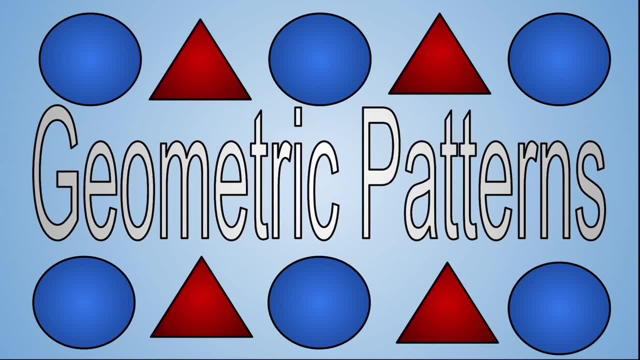 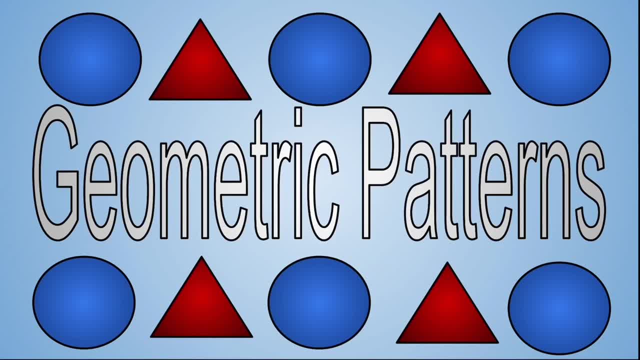 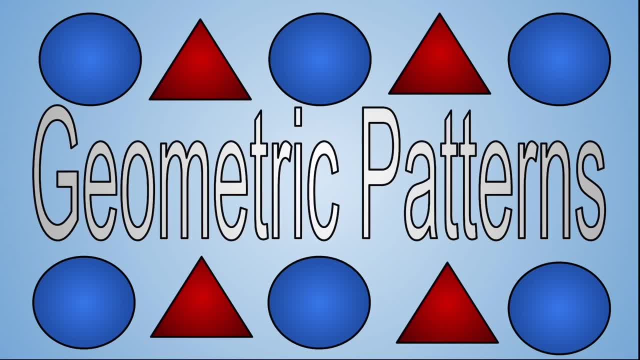 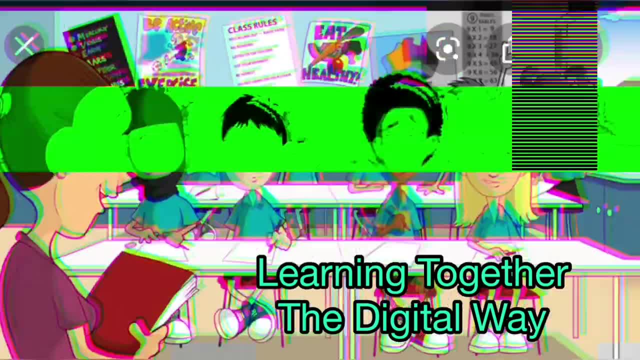 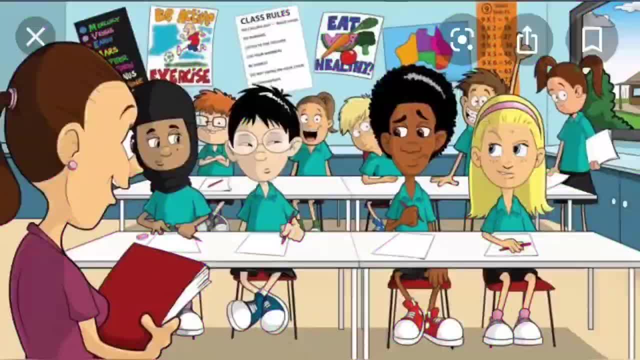